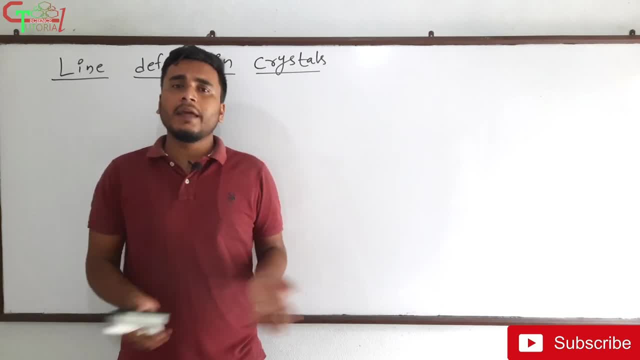 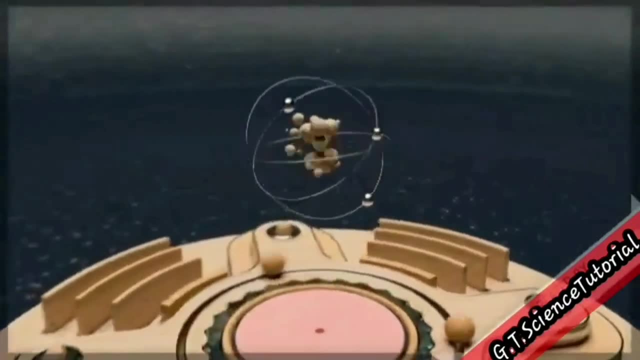 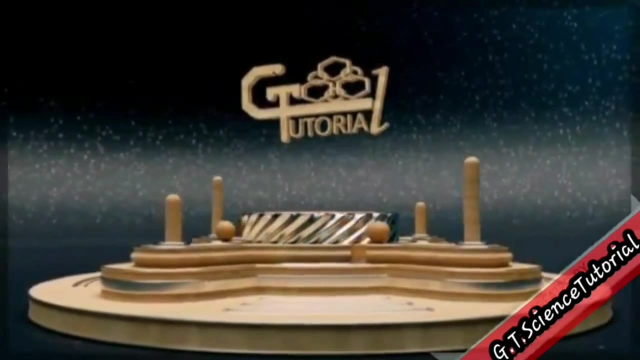 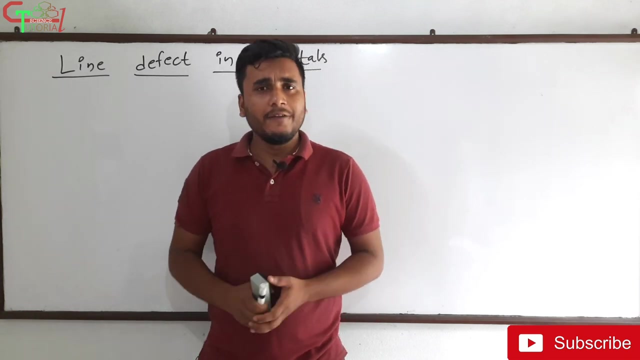 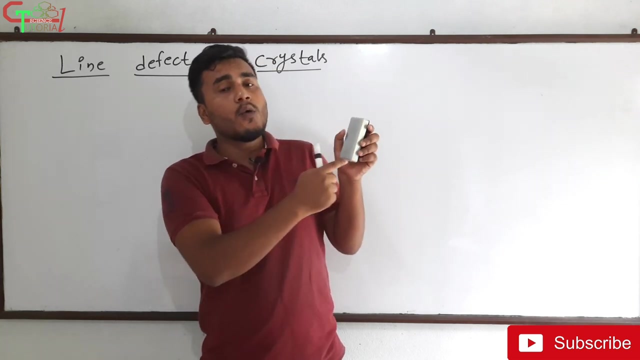 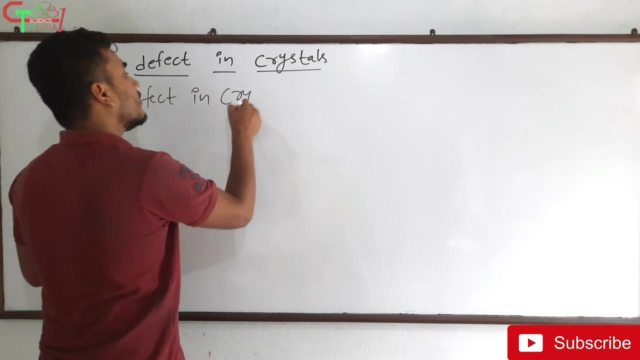 line defects are there in this video. i'm going to explain everything about that, so let's start. so just like point effect, line defects are also very common in crystals. line defect: the concept is clear from the topic itself. line means the defect will be along the whole line. so the defect, the defect in crystals, the defect in crystals. 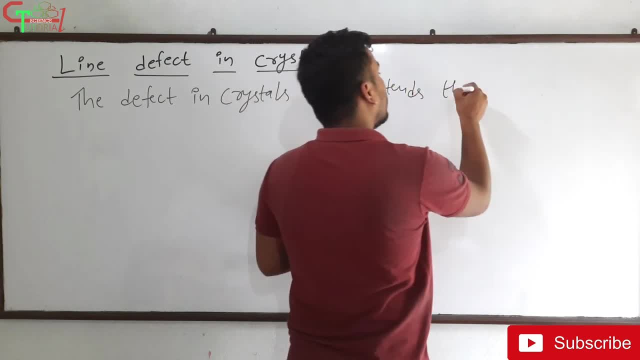 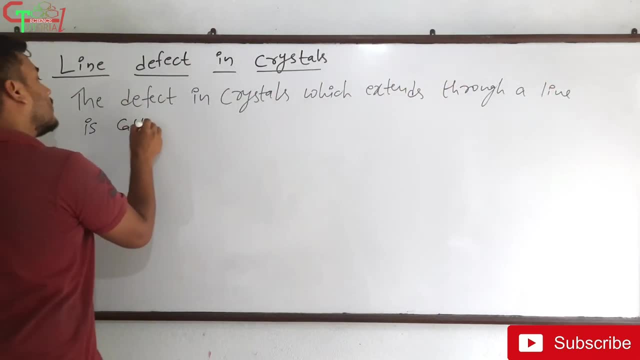 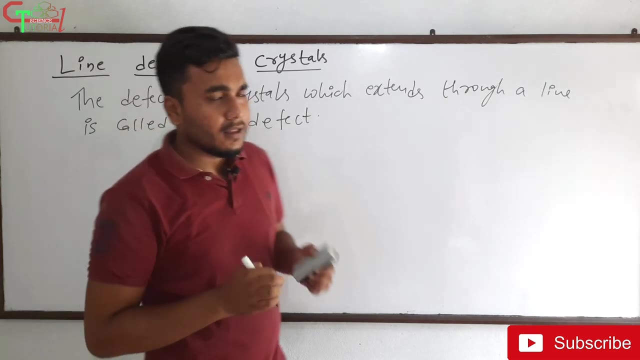 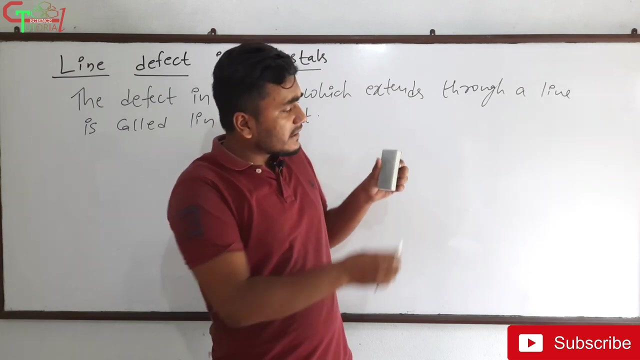 which extends, which extends through a line, which extends through a line, is called, is called line defect. so this is the definition of line defect. in this the defect is not only situated at a particular point, like point defect, but the defect extends through the whole line. that is like: 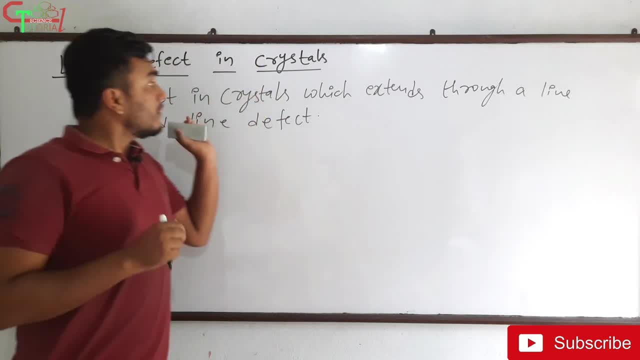 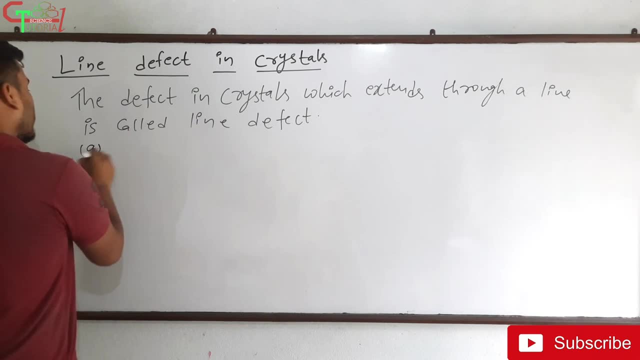 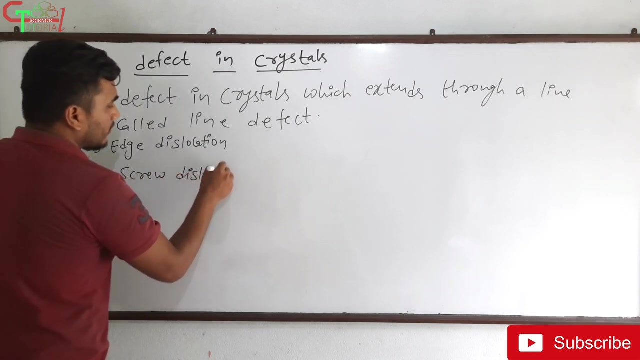 this line. okay, so this, this defect is called line defect. there are two types of line defects. they are: the first one is edge dislocation, edge dislocation and the second one is screw dislocation. the first one is edge dislocation and the second one is screw dislocation. 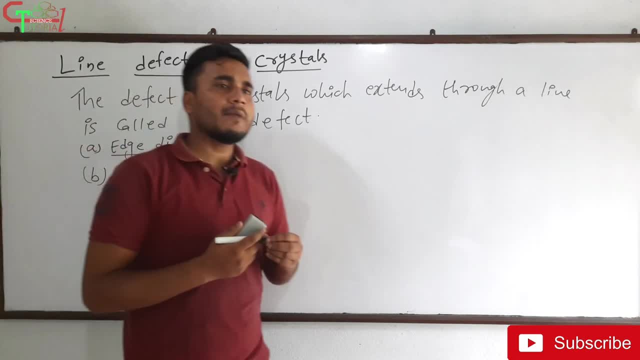 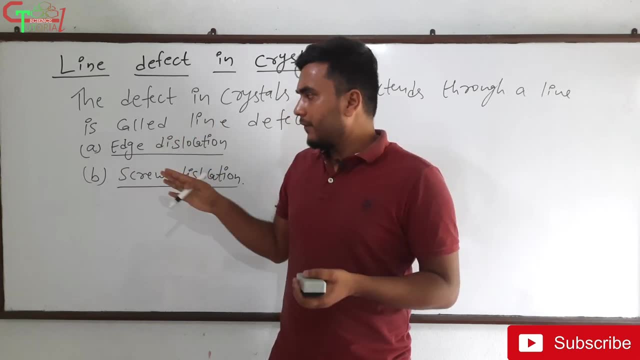 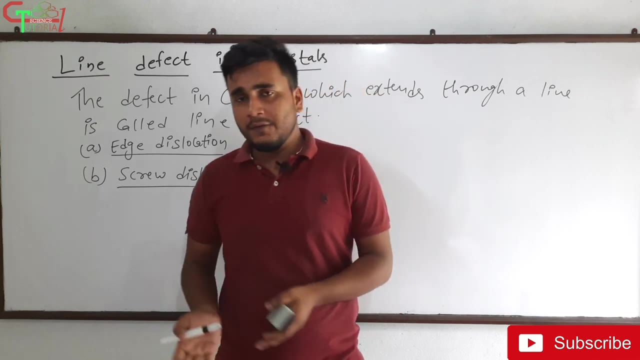 the second one is screw dislocation. there is one more type of defect in which we find both of the defects simultaneously. so in third case there will be edge defect and screw defect simultaneously. now let's see one by one. first of all we will read about s defect, then we will study about. 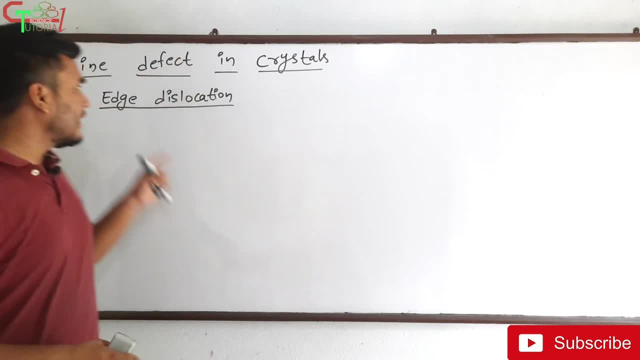 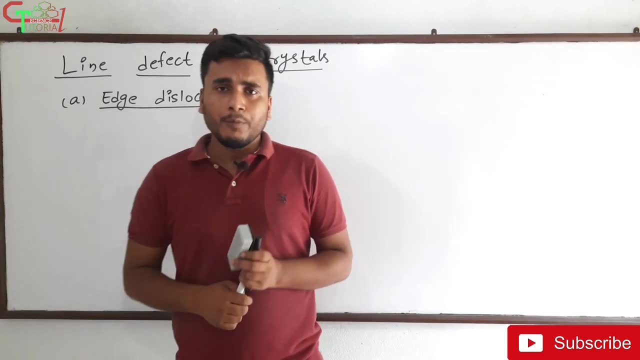 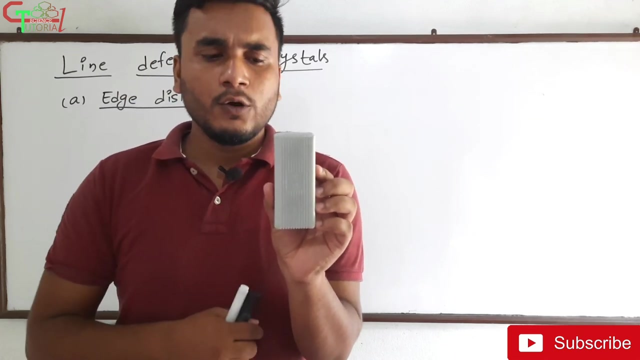 skew defect. first of all, let's understand edge dislocation. in edge dislocation there will be defect in edges of the crystal. suppose the crystal is in the rectangular form, just like this. now let's consider a scenario in which this lower breadth is constant, now this upper breadth keeps on. 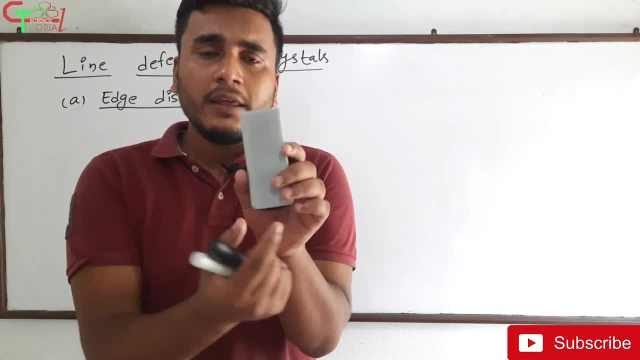 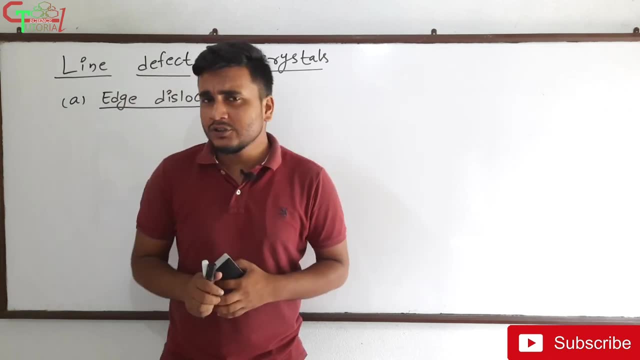 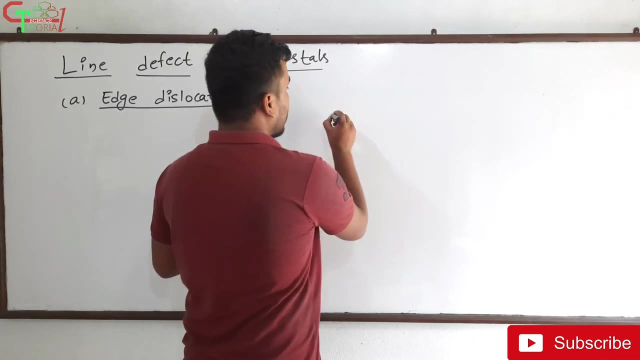 expanding and expanding. then what happens? there is the creation of defect. that's what happens in case of edge dislocation. are you getting confused? let's understand this by a diagram, which will help us understand this very properly. now look at here: the ideal crystal, or the perfect crystal, is in 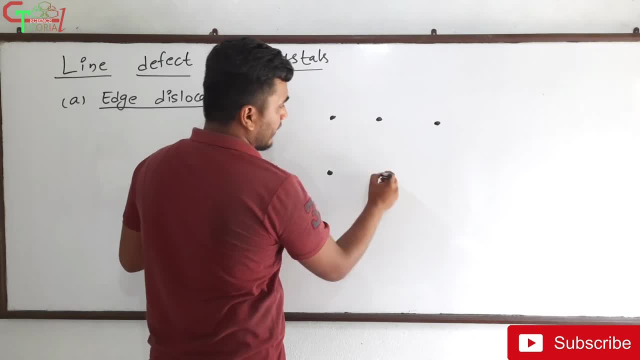 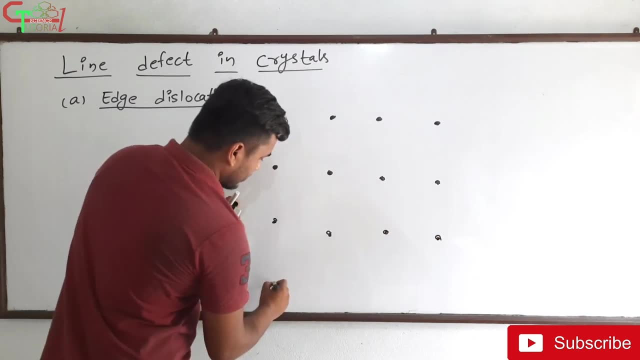 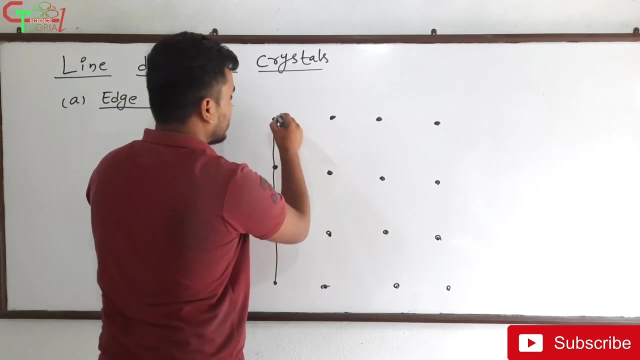 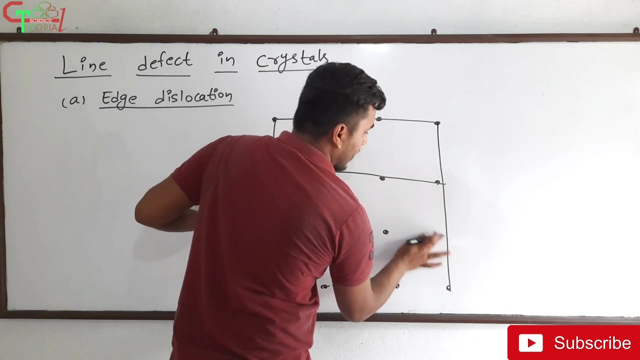 this type of shape like that means the atoms are arranged in a proper way. suppose this is the perfect crystal. this is the perfect crystal. this is the crystal structure and the atoms are in their lattice, that is, lattice side. they are in their lattice side. lattice side is like home of atoms. 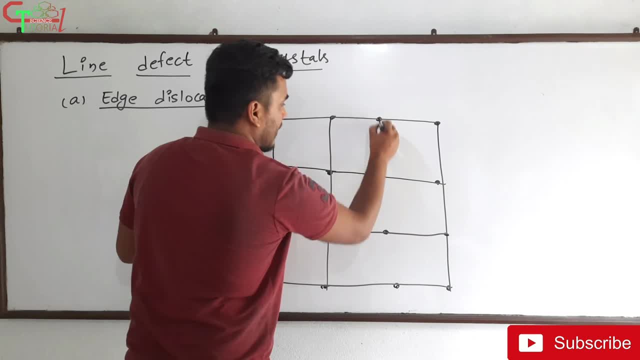 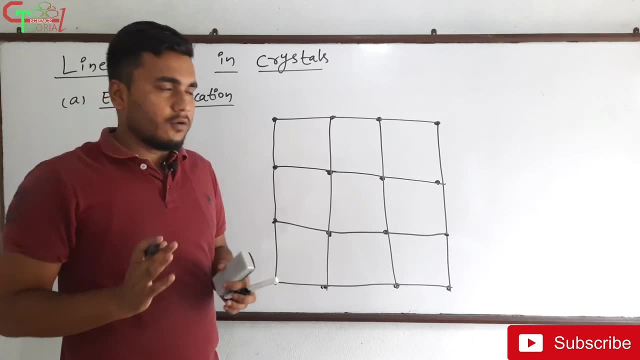 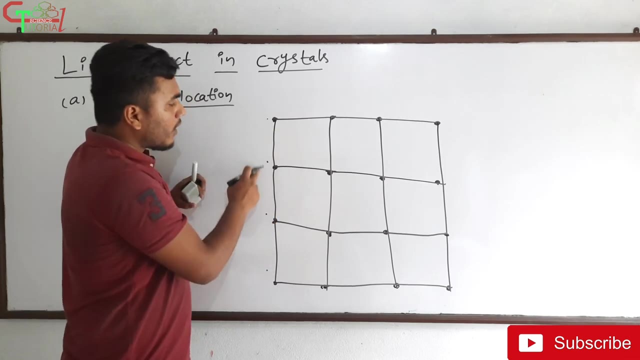 in a crystal. this is the ideal crystal. okay, now let's consider another plane, half plane. okay, how many atoms are there- one, two, three, four? in this line, that is in y axis? how many atoms are there? one, two, three and four? four atoms are there, and this is the. 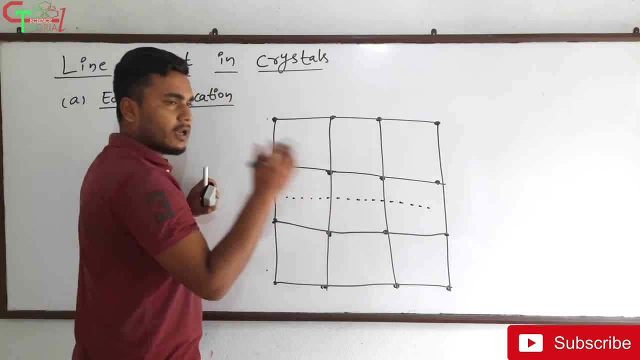 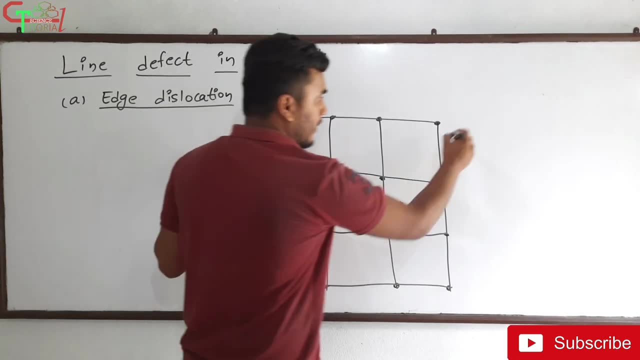 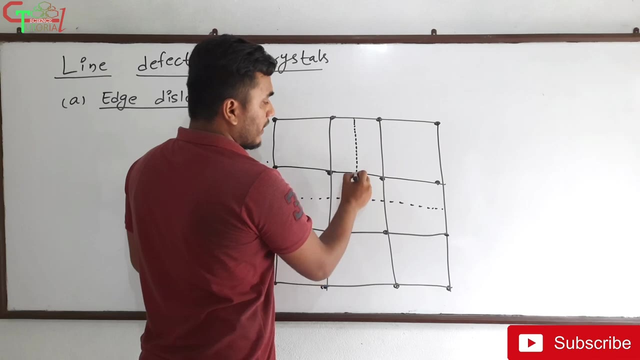 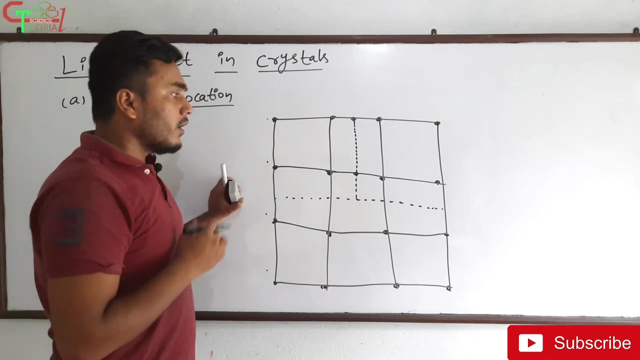 half half part of this total line right, total crystal. then let's consider a half plane in which there are two atoms. that means there will be atom, sorry, there will there. the plane will be like this: we insert a plane over here. we insert a plane over here now by inserting the plane. 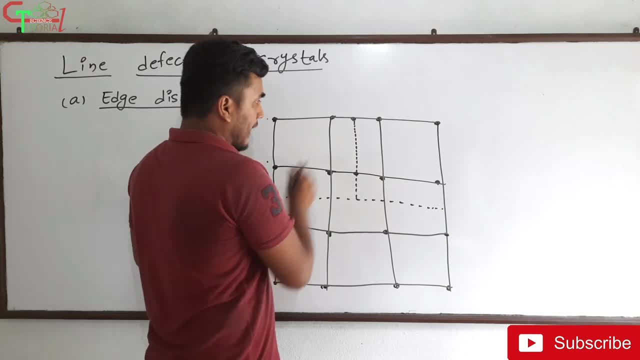 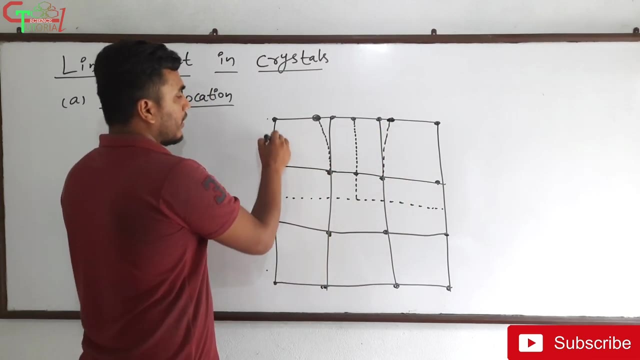 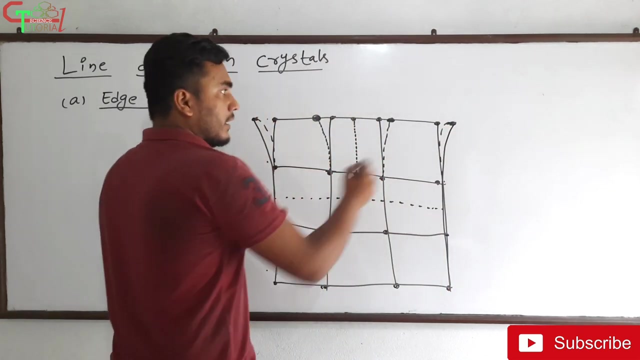 what happens? these atoms will get repelled and these atoms will change its position. this atom will come here, this atom will come here. similarly, this atom again comes here and this atom comes where here. now what happens? this is the new structure that we get. this is actually the new crystal that we get now. this 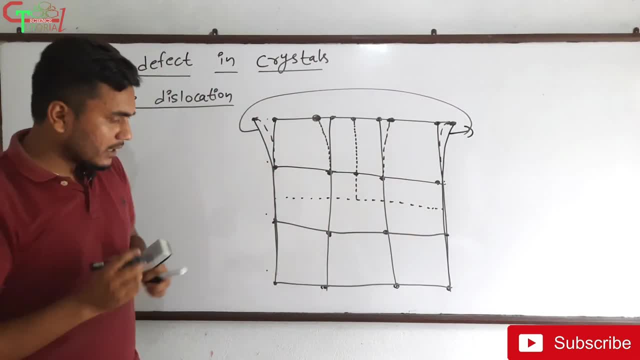 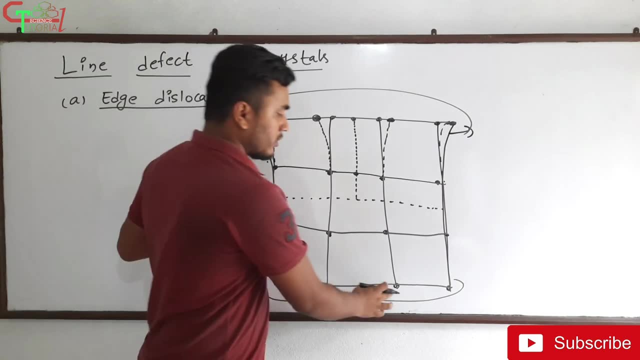 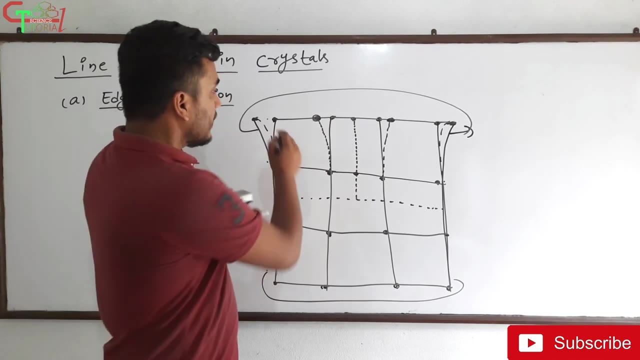 these two are the edges of the crystal. now look at here. this lower edge, or the lower breath, is constant. the length of lower breath is constant, but the length of upper breath is expanding, right, it is, uh, increasing. so this is not a perfect crystal anymore. now this defect is along the edges of 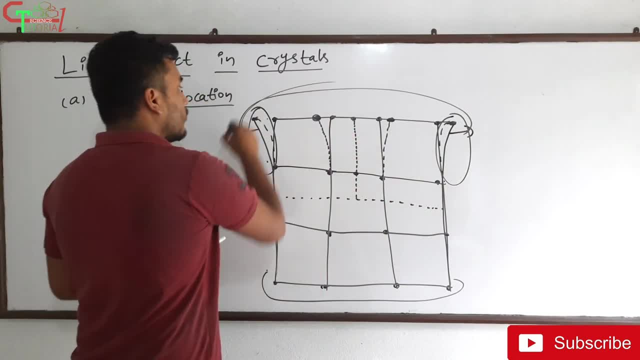 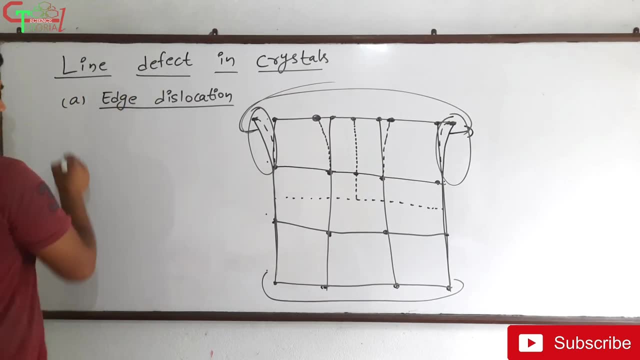 the crystal. these are the edges of the crystal. so these defects are called edge dislocation. now, if you need to write it, how do we write it? look at here: in edge dislocation, in edge dislocation, an extra plane, an extra plane is inserted, inserted in the crystal. extra, half plane, okay, extra. 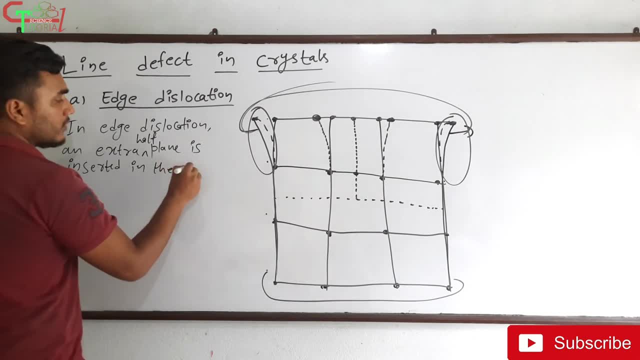 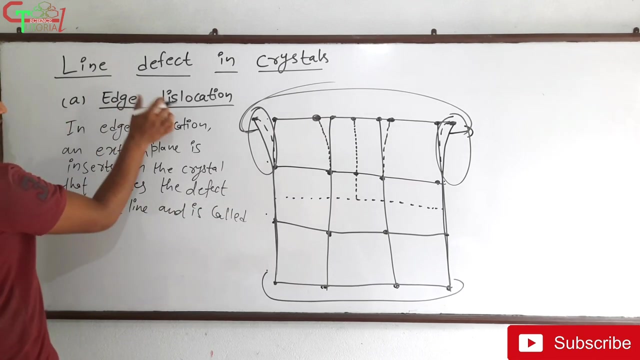 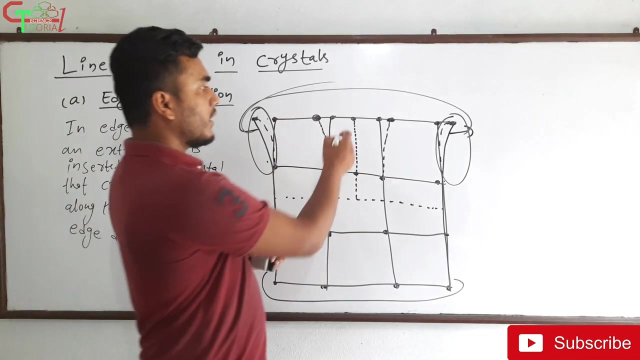 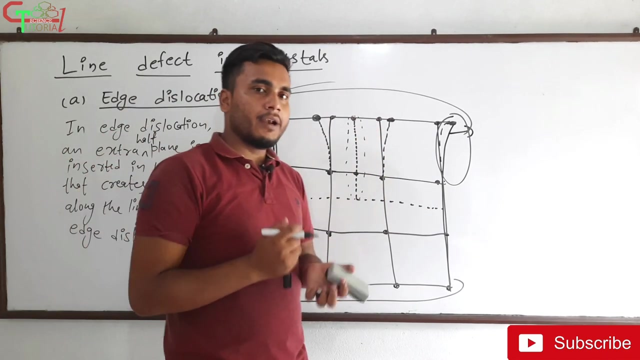 half plane is inserted in the crystal, in the crystal that creates, that creates the defect, defect along the line, along the line and is called what edge dislocation is this location? so you just saw over here, initially the crystal was in perspective of the shape, but when we insert the half explain, then the shape of the crystal is distorted. 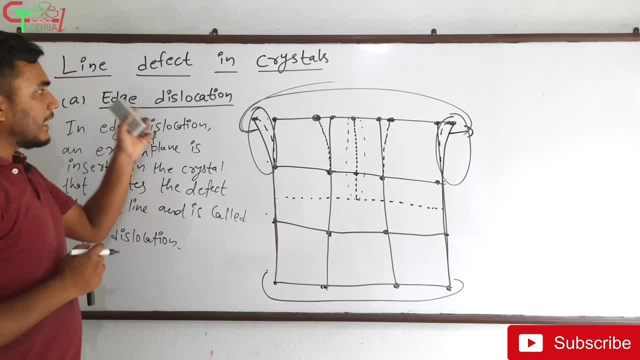 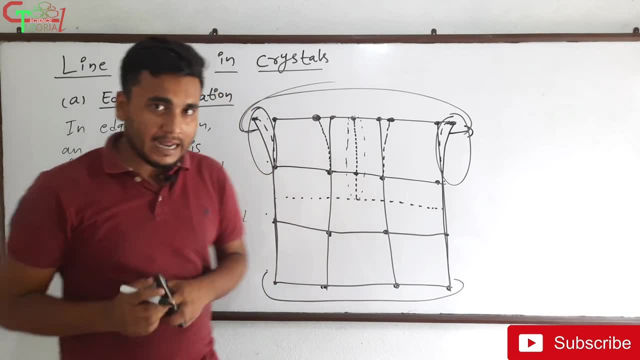 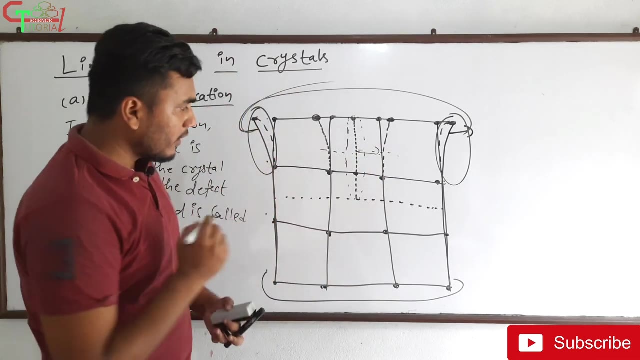 so this is the creation of defect that is called edge dislocation defect. okay, we generally find this type of form in which we get half plane in that. so this is what we call edge dislocation. now, if this moves, this is called slip. you can see over there this is. 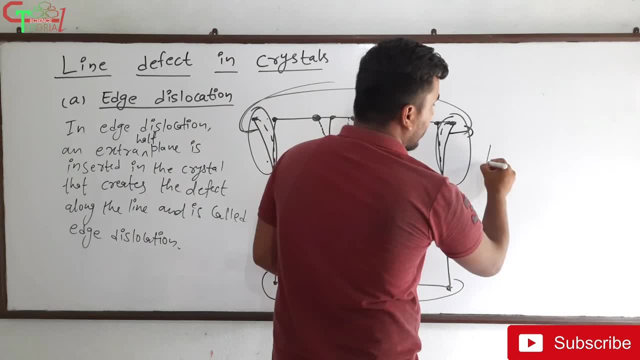 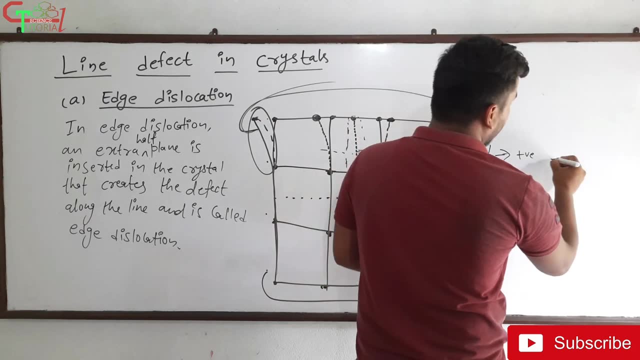 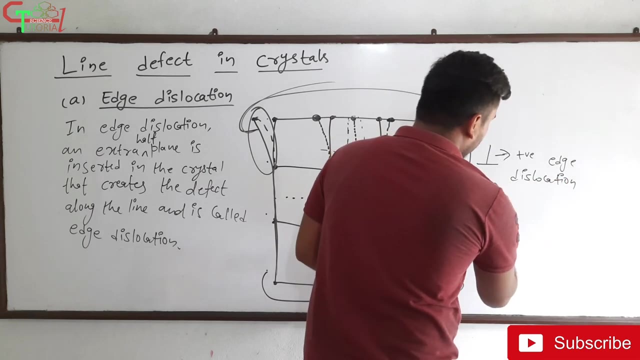 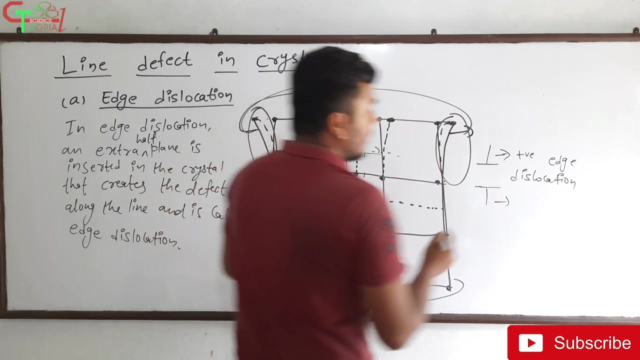 reverse t. right, this is reverse t. so if we get reverse t effect, this is called positive, positive edge dislocation, edge dislocation and if it is like this, non-diversity. if the plane was inserted from lower side, then this would be called minus, sorry, negative age. 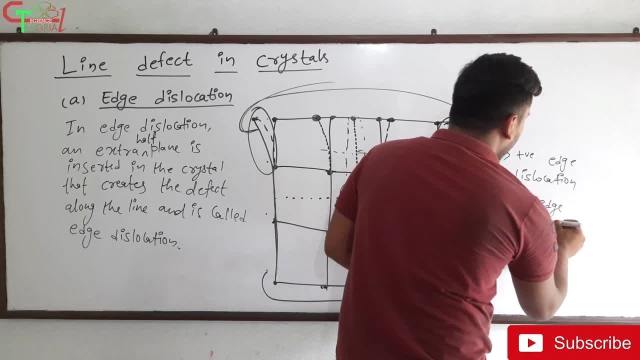 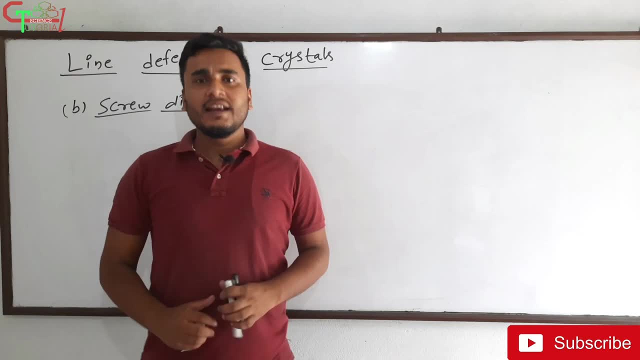 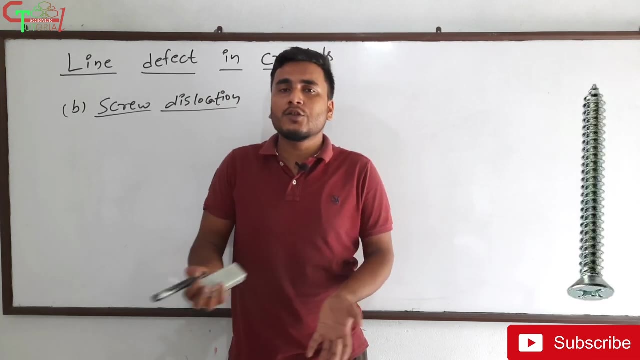 dislocation. So this is what we called edge. This is what edge dislocation actually is. Now let's see the screw dislocation. Now let's understand about screw dislocation. This defect is called screw dislocation because it actually looks like screw. Now let us consider this. duster is the. 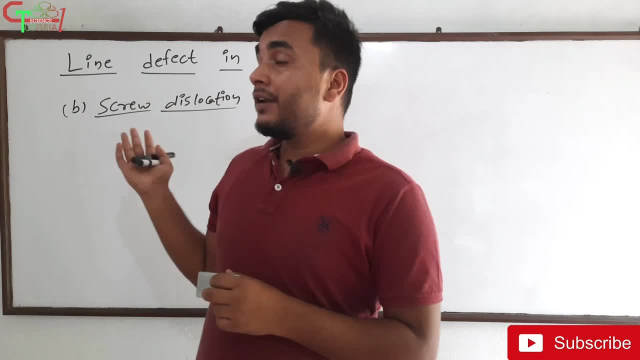 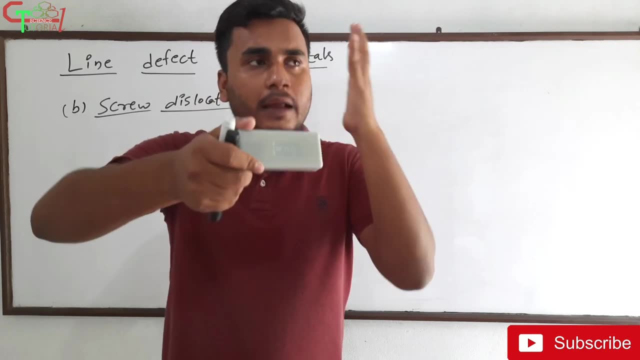 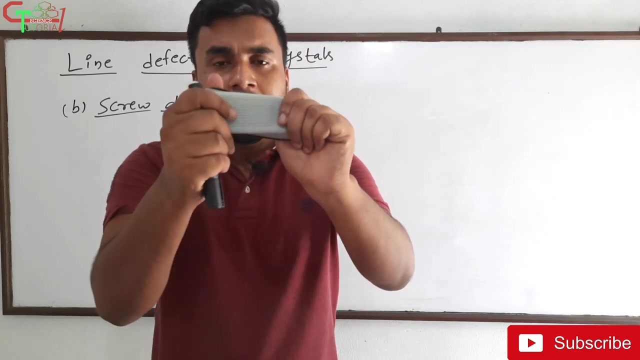 crystal. Then let me apply the force in this defect. We apply the force. Suppose I am using my right hand to apply the force in this direction, I am using my left hand to apply the force in another direction, That is completely opposite direction. Then what happens? This is rotating. 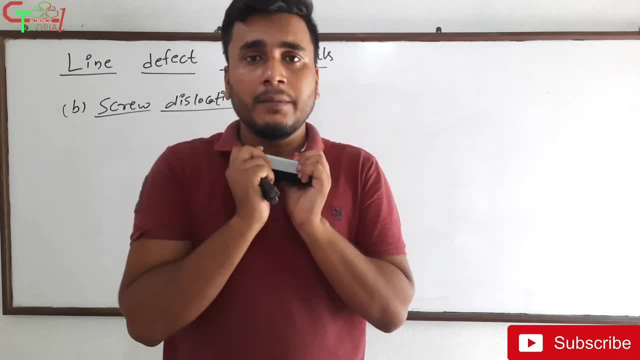 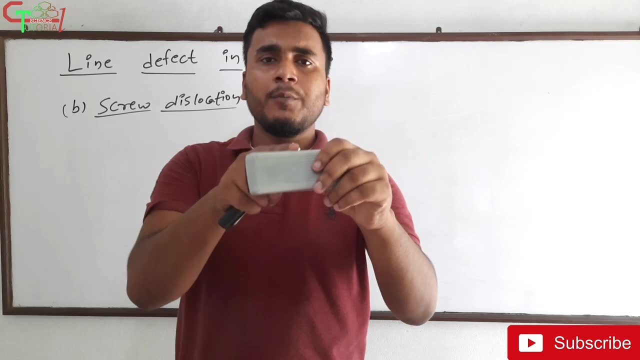 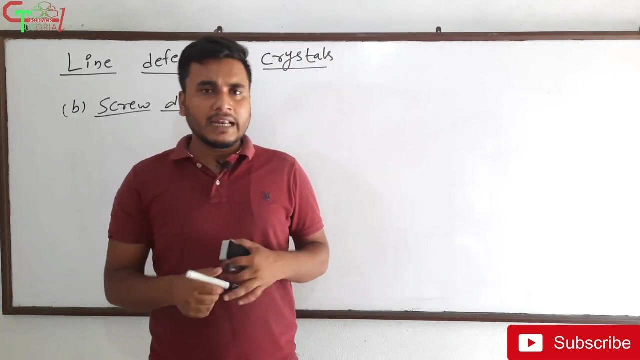 right Now this is hard, So it does not feel any effect. But in case of crystal, what happens? when we apply the force in opposite direction, The atoms of this portion, the middle portion, actually gets displaced and change its position, So that creates the defect. Now let's understand that. I am using my right hand to apply the force in this direction. I am using my left hand to apply the force in this direction. That is completely opposite direction. Now let's understand that I am using my right hand to apply the force in this direction. That is completely opposite direction. 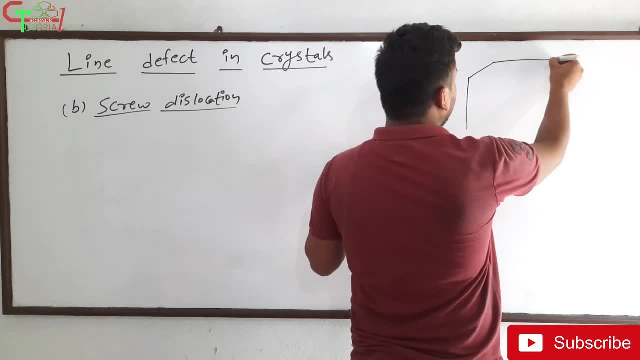 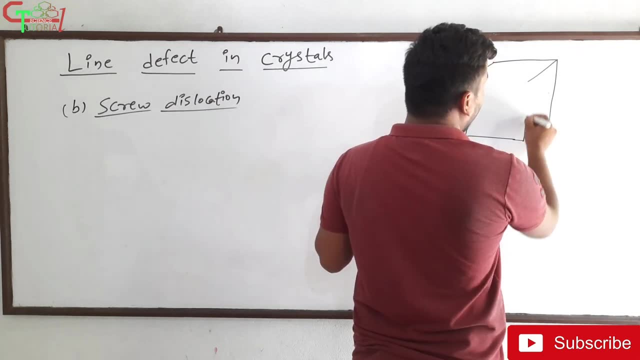 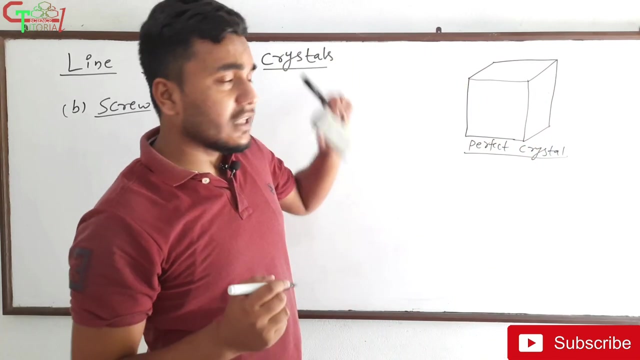 This is the perfect crystal that we actually found that we need to get. This is the what Perfect crystal. Okay, This is the perfect crystal. The crystal should be in this structure, But no, Due to the thermal effect, the crystal is not in this defect And because of the stress, the 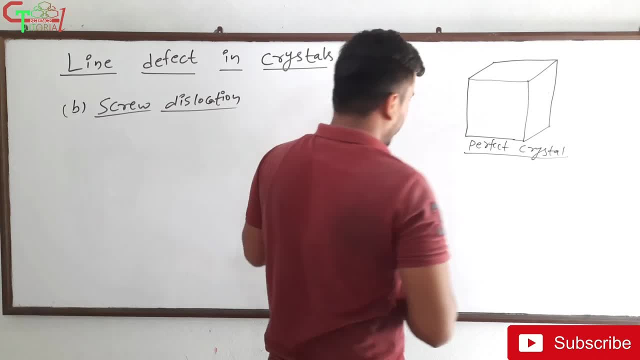 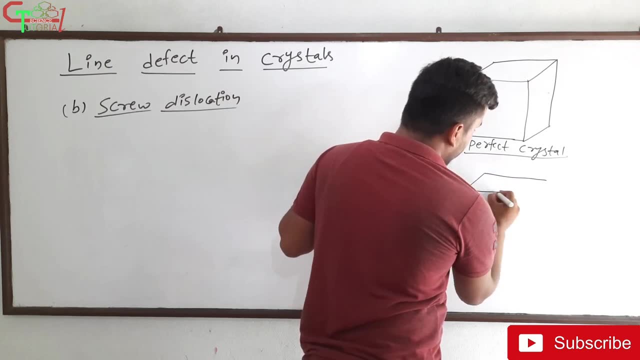 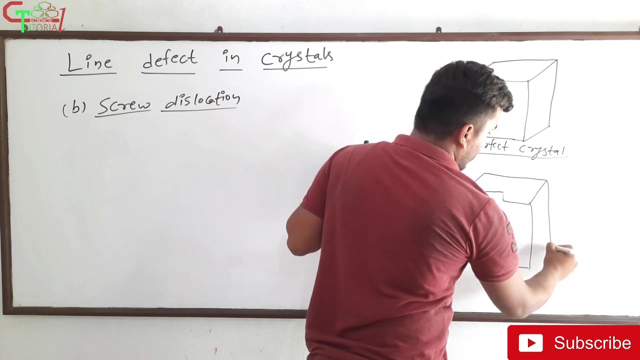 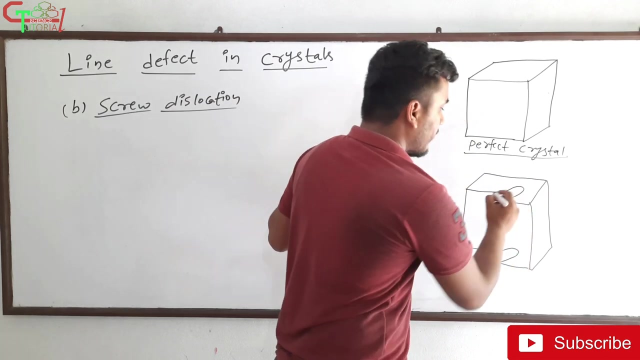 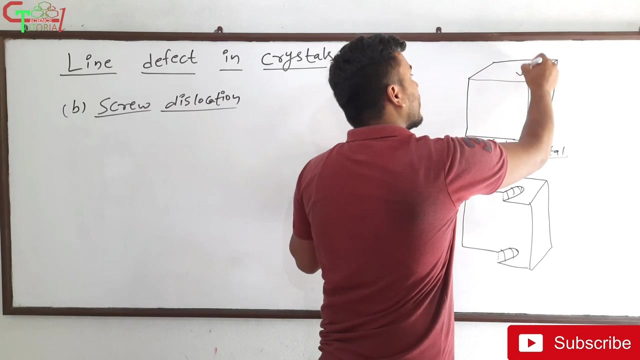 defect is produced in the crystal, now in screw defect. what happens now? look at here. the crystal gets a defect like this. okay, you can see over here- i've just made the diagram of it- what actually happens when we apply the stress in opposite directions: from here downward, from here upward. then we get: 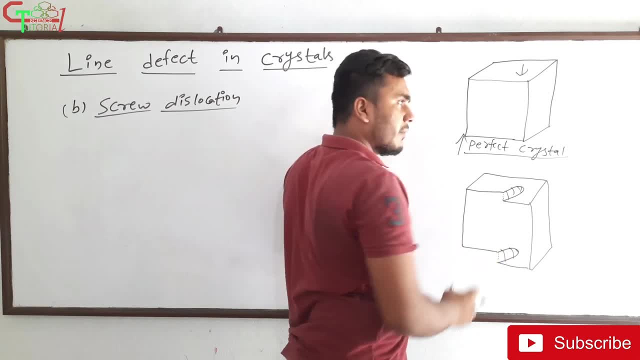 this type of form, this type of structure or this type of diagram, in case of a structure, of this type of structure, and we get the form like this and we get the form like this and we get the form like this of crystals. here, this part, from this part, the atoms have been moved, the atom.